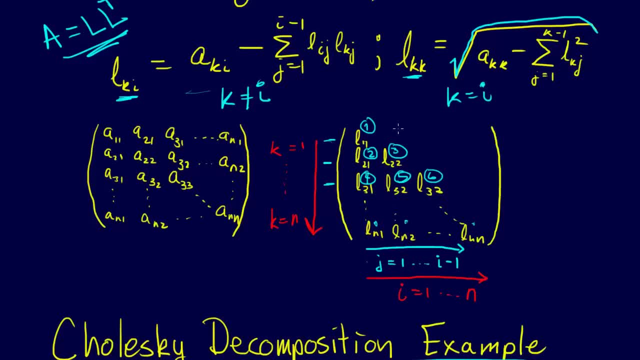 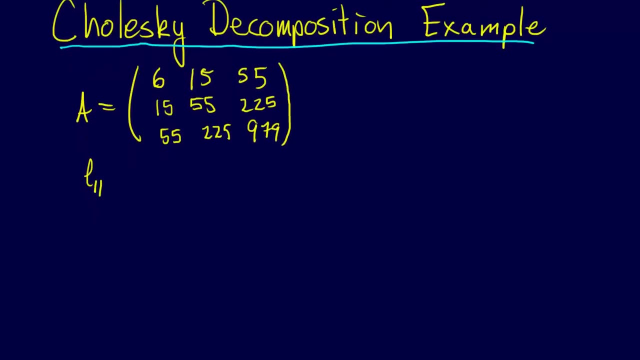 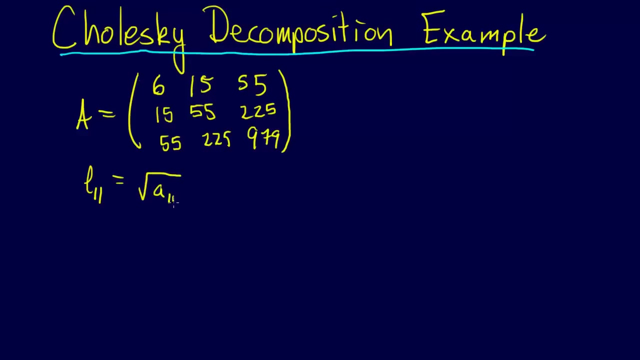 Well, this summation actually moves over here and we're still in the first row, and so there is no element here, And so L11 is just going to equal the square root of A11.. So L11 equals the square root of A11.. 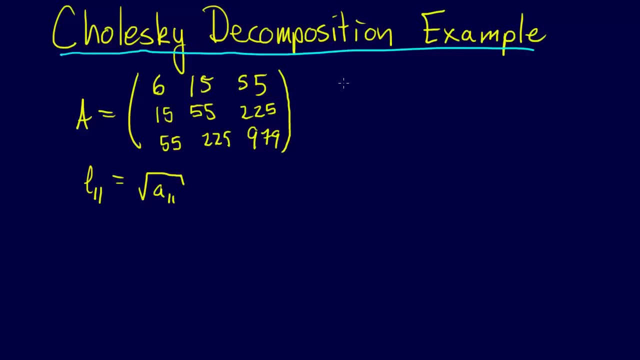 All right, good, So we've done that one, and if we look, let's say, L equals, so we've got it here And to give a number to that, that's equal to then the square root of 6. Which is equal to 2.4495, and so we could just write that 2.4495 right here in the first entry of our matrix code. 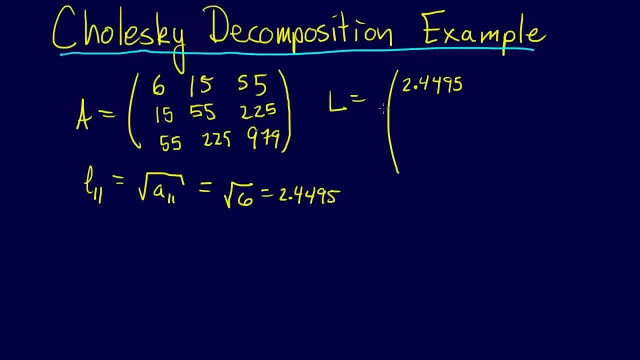 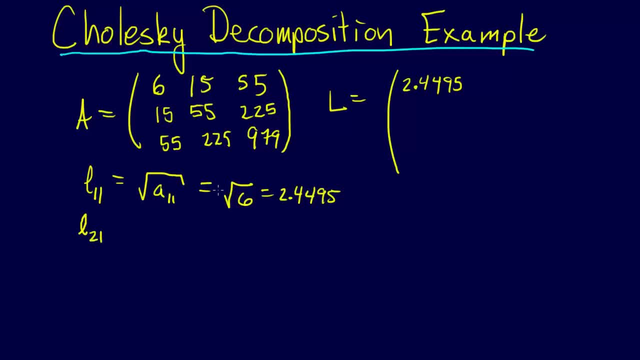 That's going to be L21.. So that's K equals 2.. So this is K equals 1, I equals 1.. So this is K equals 2, I equals 1.. All right, so K equals 2, I equals 1.. 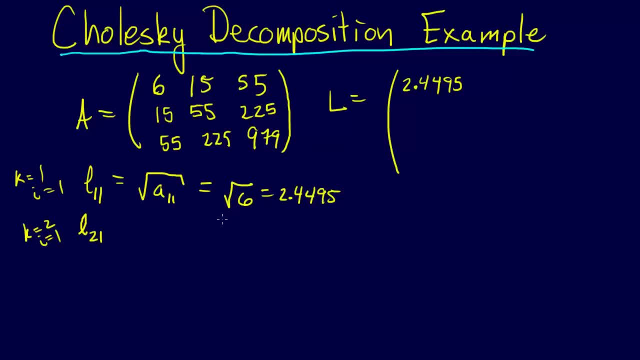 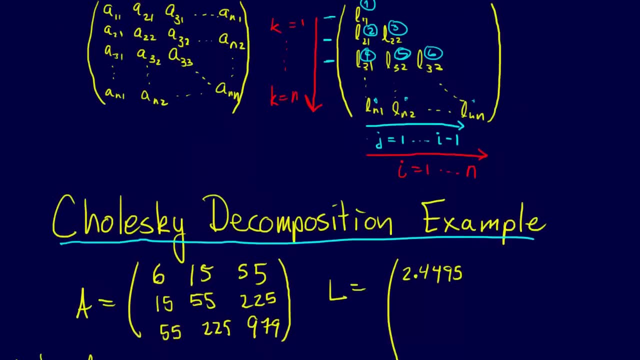 L21 is going to equal, then our: Okay, we just use this, We just use this other equation here, so we're going to use: Sorry, I keep moving back and forth here. Maybe I should copy this down. Yeah, let me do that. 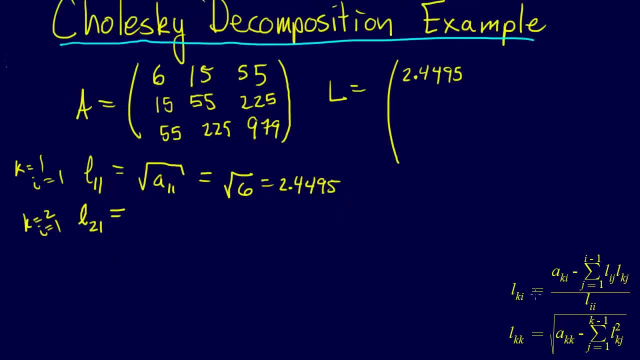 Well, let me do that and I'll come back. All right now we've got them here And if we look we're here, We're on this second entry. so that's going to be the A that we're going to base it on. 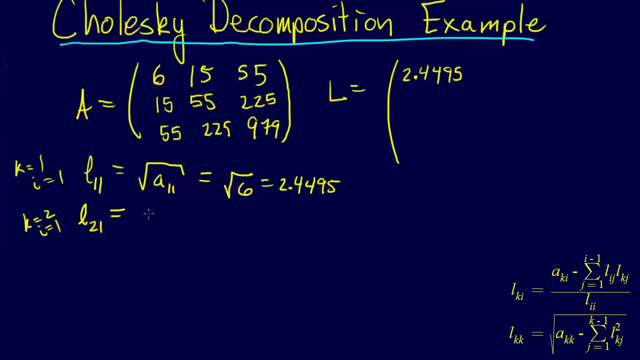 It'll be AKI, So that'll be 15.. I'll just write 15.. 15 over minus. So normally it would be minus here. but if you look, J has to start at 1 and go to I minus 1,. 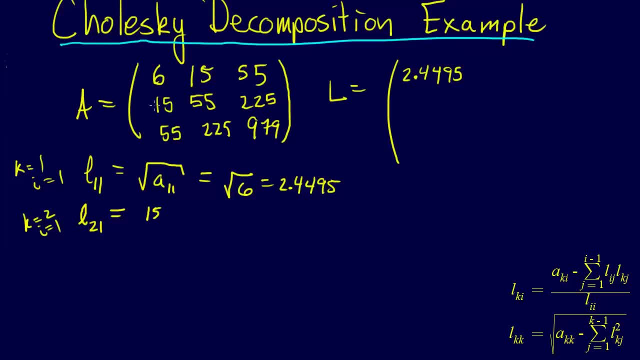 and our I is only 1.. So we're in this first column and so we're not going to move over 2 here. That doesn't mean anything, And so we don't have to do anything with this term. That doesn't come into play. 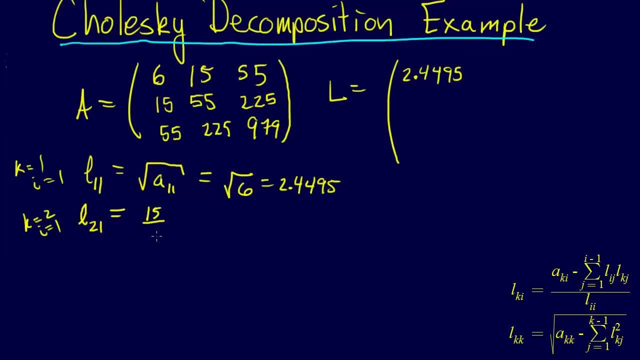 So then that's going to be divided by LII, That's going to be, Well, not 6,, but the square root of 6,, which is 2.4495.. And that is 6.1237.. All right, so then we can move. 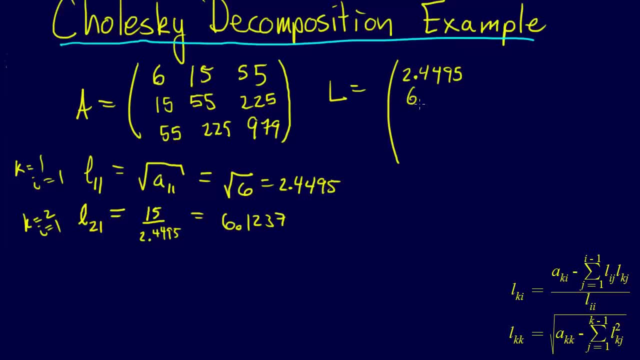 So we've done this entry, so we've got 6.1237.. Now we're going to move to this, This other diagonal entry, and because we're on a diagonal entry, we're going to use this second equation, And so that's going to equal 2.. 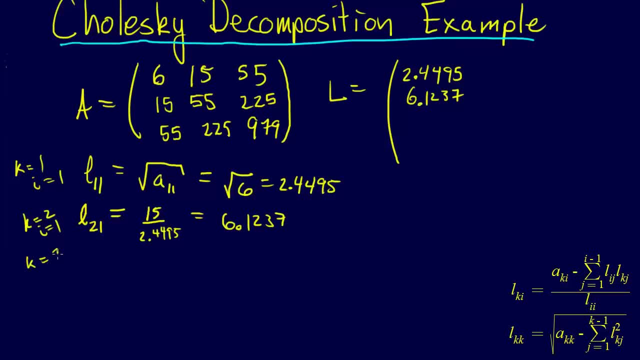 So we have K then equals to still 2, but our I is equal to 2 now, And so we're going to say L22, and that's going to equal. Well, it's going to be based off just like they always are at A22. 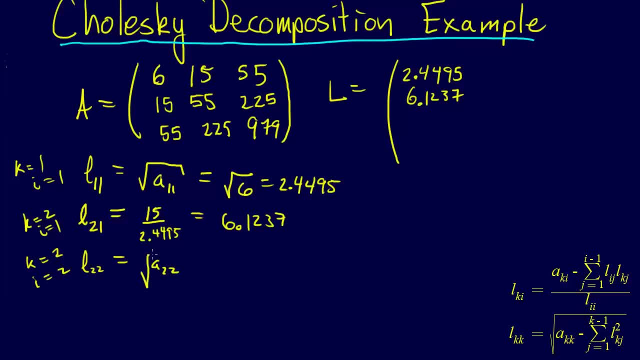 So it's going to be A22, and it's going to be the square root of this minus Sum sum here. Okay, so we're summing from: J equals 1 to K minus 1.. Really, what we're doing is we're summing up these terms squared. 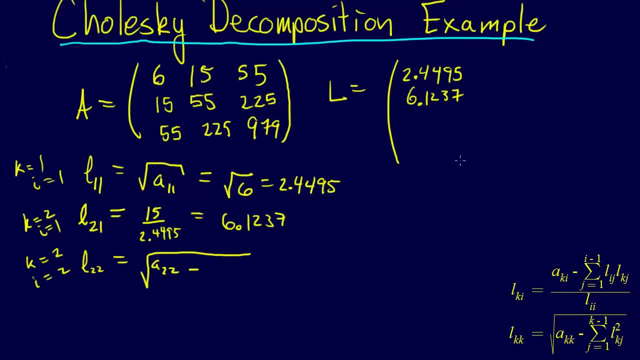 so it's going to be that term squared, because that's the only one to the left of it. We're summing up all the terms to the left of it in the L matrix, So that's just going to be that squared. So 6.1237 squared. 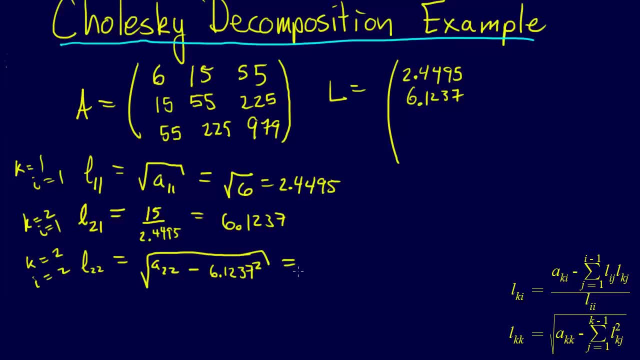 And that is going to equal 4.1833.. This is 15 here, right, Or not 15, but 55.. See, 55?? Yeah, 55, right here, 55.. That's the entry that we have: the A22 entry. 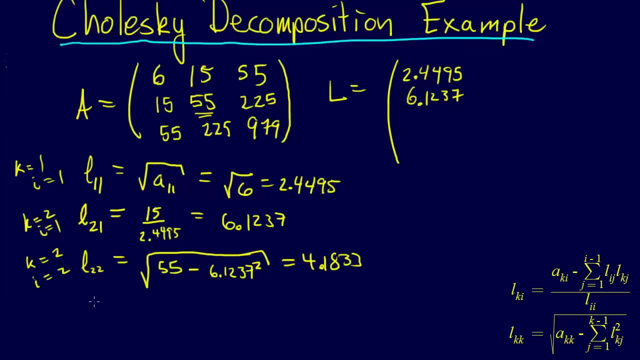 It's 55 here, Okay, so we're in good shape there, And so now we have 4.1833.. Now we can move down to the next row, because we're completely done with this row, right? Because there's zeroes up here, so we don't even have to worry about those. 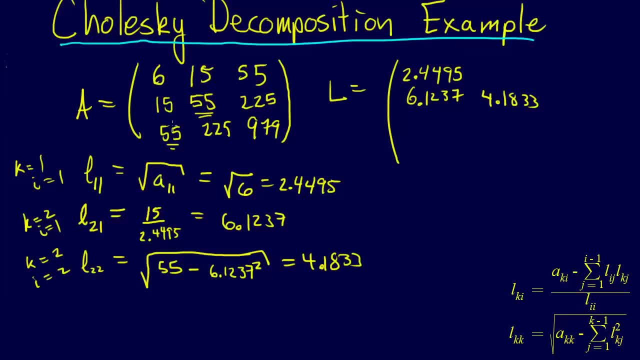 So it's going to be based off of this, And it's also not a diagonal entry, So we're going to use this first equation, And so then the first term is going to be: so L- so this is K- equals 3.. 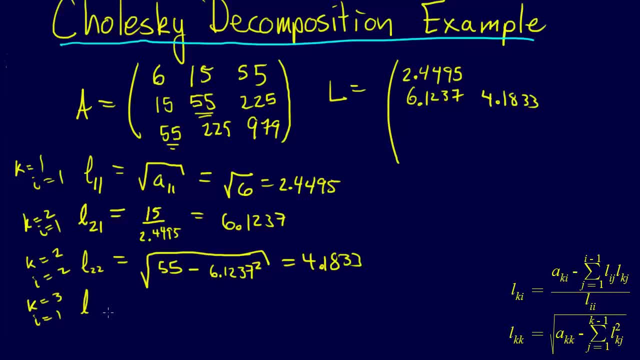 I equals 1.. Start I over again. So L31.. 3, 1 equals, and it's not going to be a square, it's going to be 55.. Yes, 55. That entry is going to be 55 minus the sum of all the previous elements. 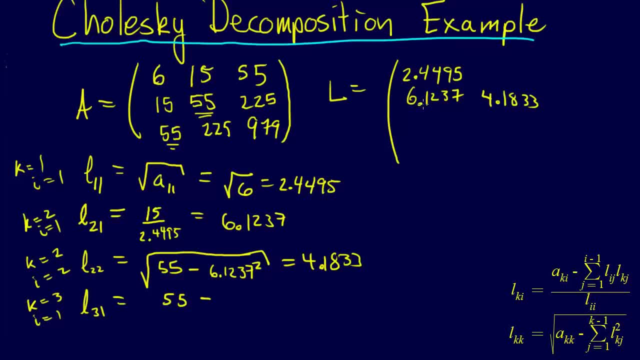 And there are none here, none to the left of it, And it's really the Ls that we're summing. So there's none to the left of it, because it's right here. This is where it's going to go. 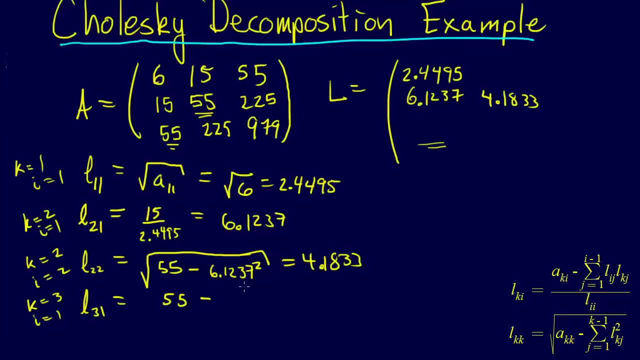 Divided by Li. So that's that entry. So divided by so minus zero, really Divided by 2.4495.. And that is going to equal 22.454.. Alright, So we can keep moving through. I'm going to move down a little bit here. But we can put that in here as well: 2.4495.. All right, So we can keep moving through. I'm going to move down a little bit here, But we can put that in here as well: 2.4495.. 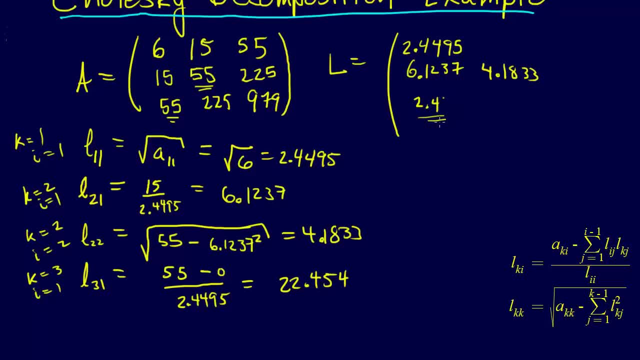 So that's going to equal 22.454.. Alright, So now we moved over, Now we're on this entry here, So that's going to be L32.. Because we have: K equals 3.. I equals 2.. Why did I set it to 2?? 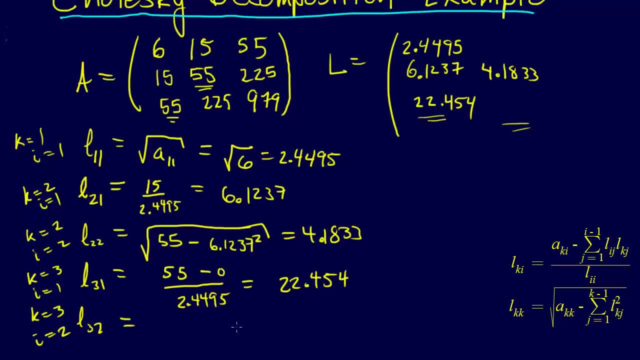 But I wrote a 1. So that's going to equal. then That will be based on that A right, This A the corresponding A entry. So it will be 225 minus again the sum of all the entries to the left. times, IJ times, KJ. 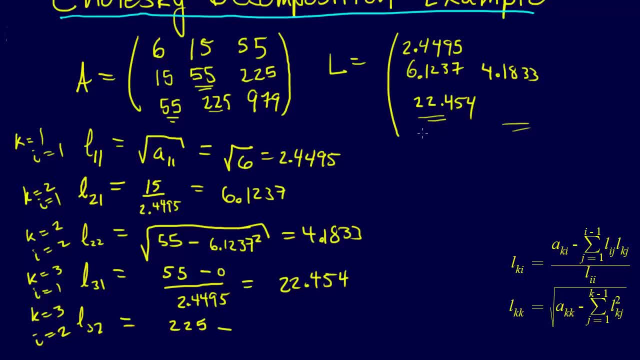 So that's going to be 225 minus L IJ times KJ. So the IJ, that will be this entry here, And then the KJ entry will be this entry here. So that will be minus. And see, there's just the two. 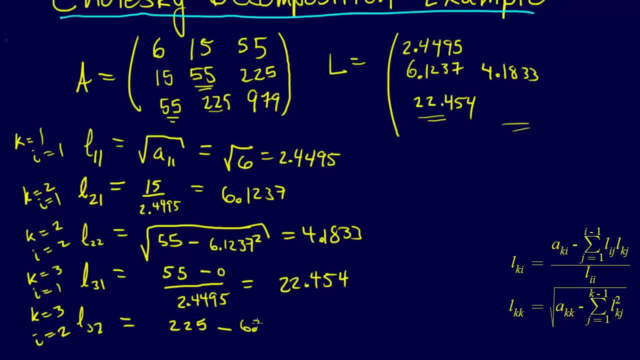 So that's going to equal 22.6.1237 times 22.454.. And that is going to. Let's see, Do we have to divide it by something? Yeah, L, I, I And I is 2.. So we have to divide it by. 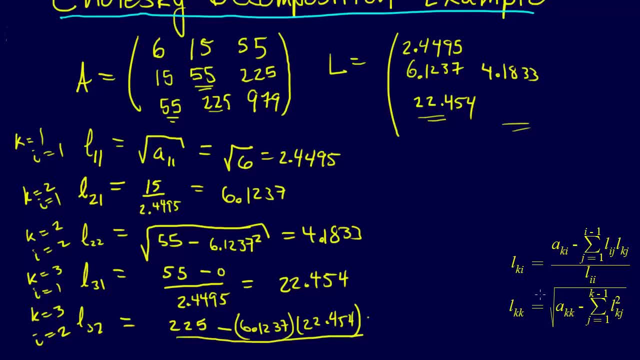 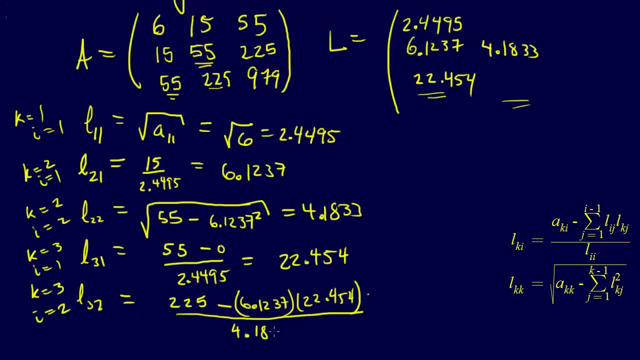 This guy all over- I'm going to slide down here a little more- All over 4.1833.. And that is going to equal 20.917.. So we can put that in here: 20.917.. We're on the home stretch. 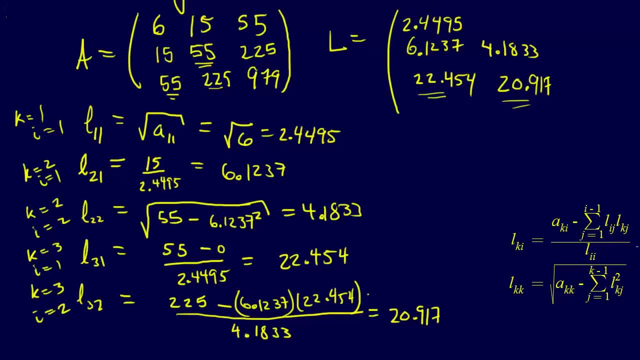 We got our last entry. It's going to be a diagonal entry, So we're going to take the square root And see, yeah, So you notice, here we got this. This is going to be This is squared. And see, this is sort of similar. 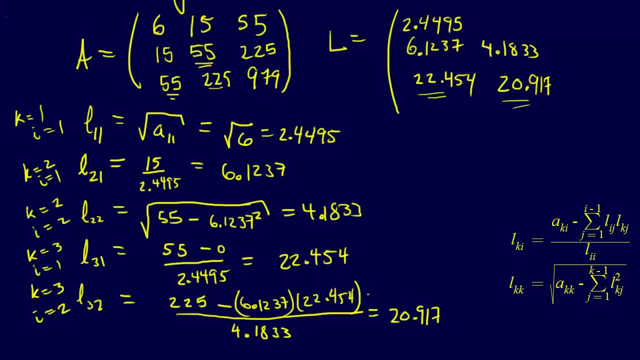 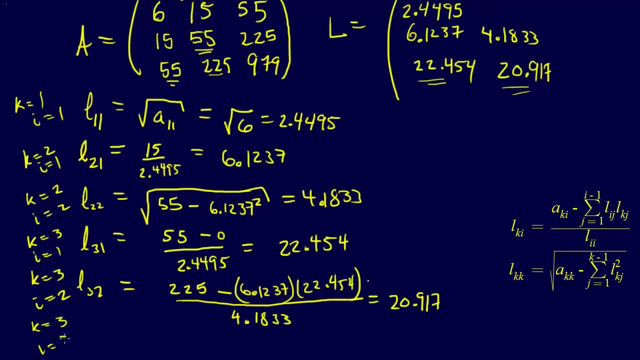 It's not squared, But it's going to be one element times another, So it's still the product of two elements Interesting. So this is: K equals 3.. I equals 3.. So then we have L33 equals AKK. 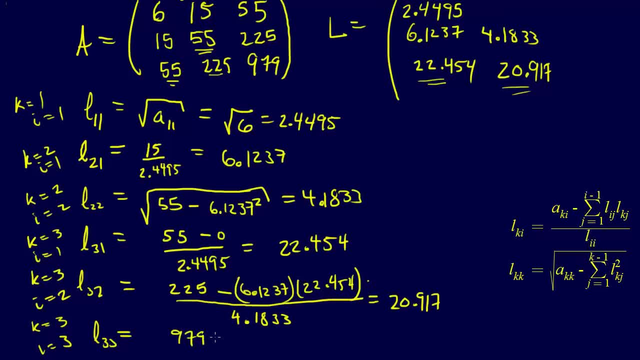 So that's going to be 979.. 979.. Minus- And it will be the square root of all this- Minus, The sum of L squared, LKJ squared, So K is 3.. And what is J? 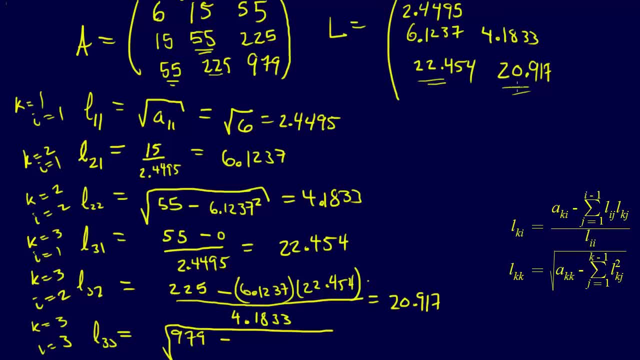 Well, J has to move all the way across here, So that's going to be A33.. Yeah, So we have that 979 minus L31.. So we'll take the first entry. So 22.454 squared Minus the square root of this squared. 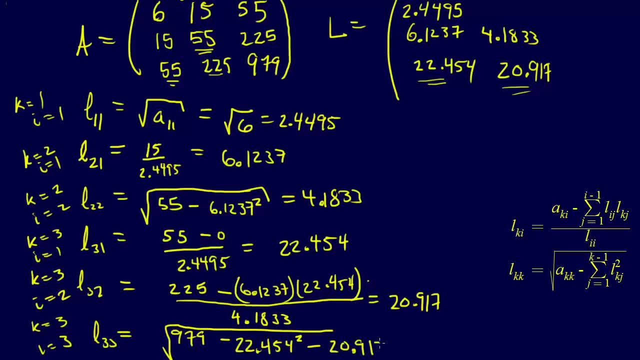 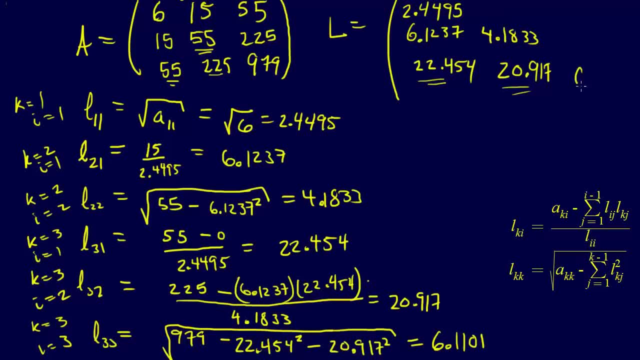 20.917 squared, 20.917 squared, 20.917 squared, 6.1101.. So we can put that 6.1101.. And we're done. So there's an example of Cholesky decomposition. 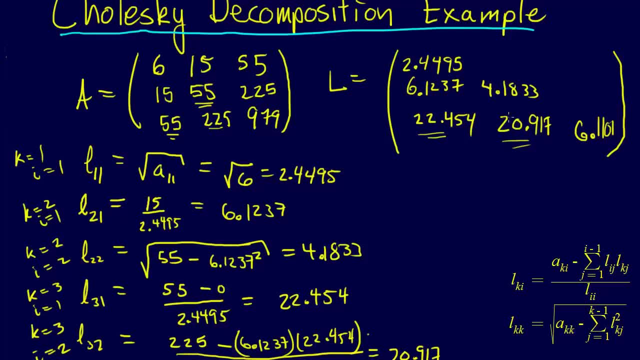 And that is our Sort of like, our matrix, square root. 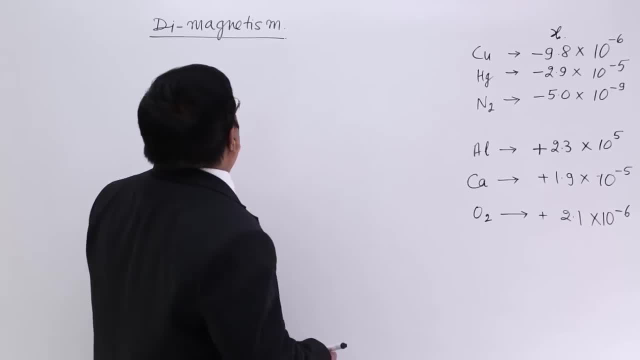 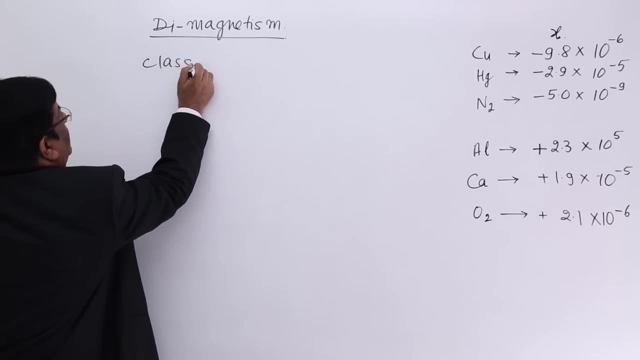 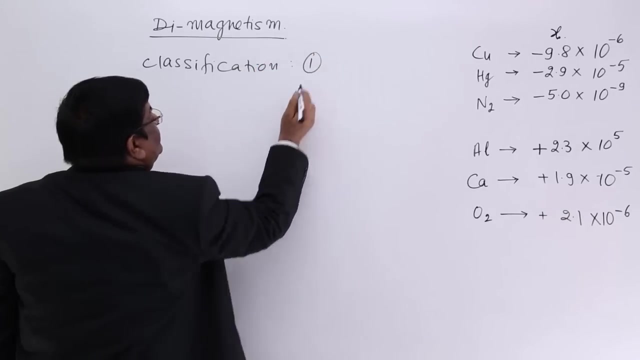 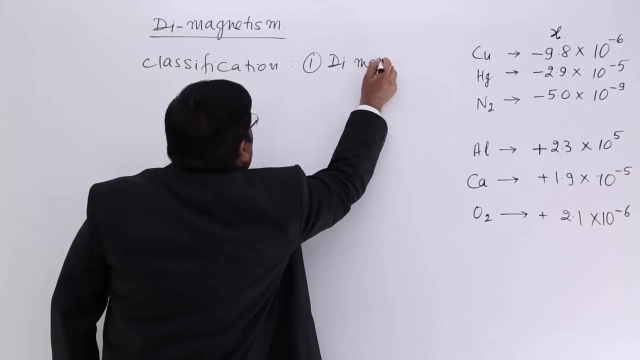 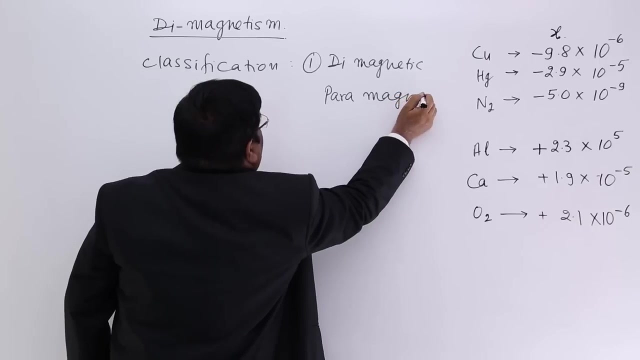 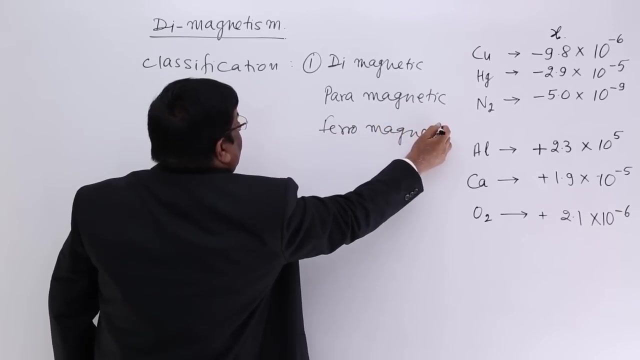 Now we are coming to classification of material with reference to magnetization. There are three type of material, three categories of material: One is Dimagnetic, other is Paramagnetic and the third is Ferromagnetic. First I will take up Dimagnetic.